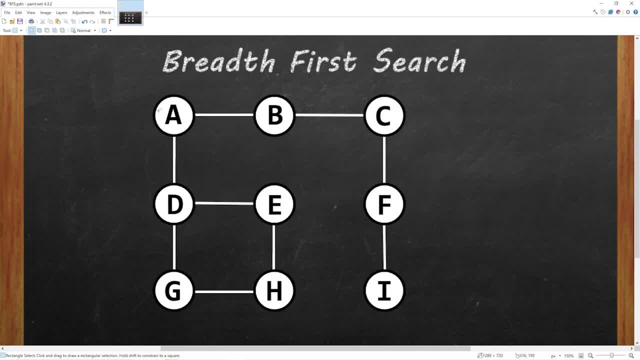 topic on depth first search, we would navigate a graph one branch at a time. But in a breadth first search approach, we would navigate this graph one level at a time. So let's begin at node A and we are attempting to travel to node I. Instead of a stack, we'll use a queue: All. 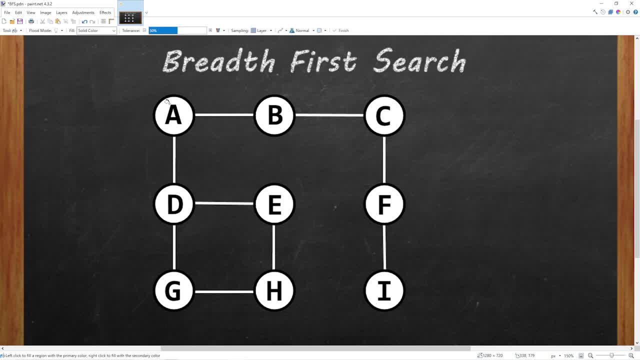 unvisited nodes we will add to the queue. So we're currently at A. We'll add that to the queue. Then add any unvisited adjacent neighbors to the queue as well. We have both B and D as neighbors, So we will add these to the queue. Then add any unvisited adjacent neighbors of nodes B and D. 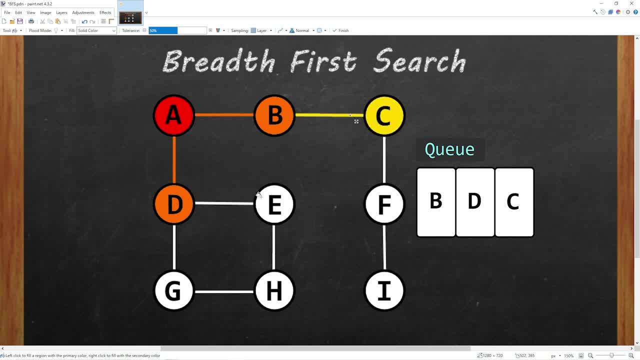 That means we will add C, E and G And for the next level we have F and H And lastly I. So that is a breadth first search approach. We will navigate a graph one level at a time, using a queue rather than one branch at a. 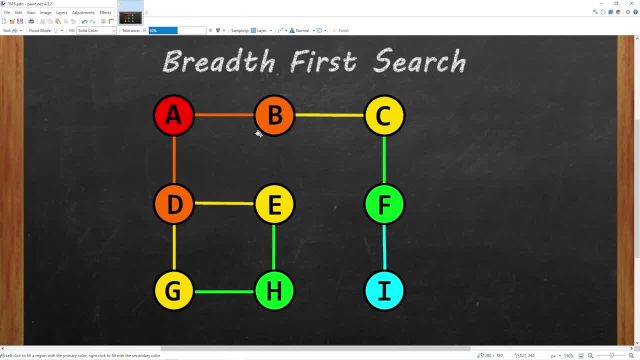 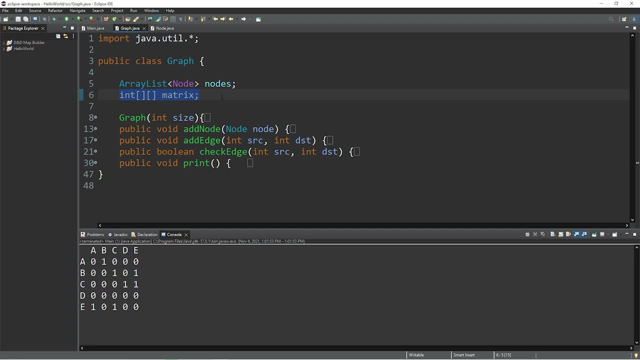 time using a stack, like with depth first search. Let's implement this in code now. Okay, everyone. so in my graph I'm utilizing an adjacency matrix, So I have the same code from the previous few videos And we have a node class that contains: 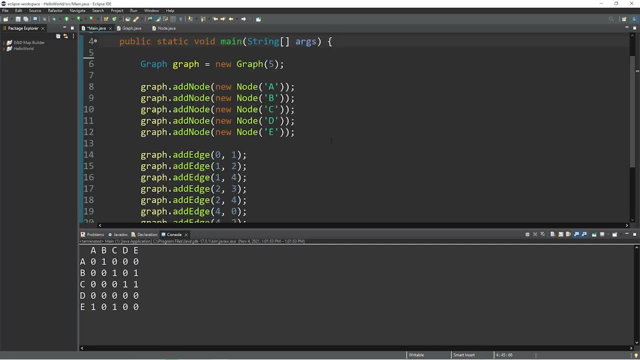 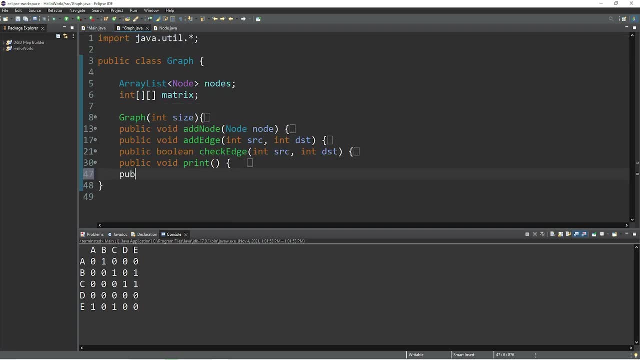 some data And I went ahead and populated this graph. already It's the same data from the previous few topics. Heading to our graph class, let's create a breadth first search method, Public void- breadth first search And we will take an integer named source. 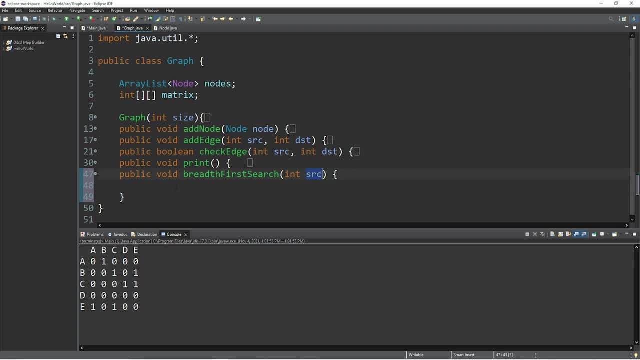 This will be the index of the node we would like to begin searching at. with a breadth-first search. we can utilize a queue, So queue. we will store integers, these will be indices and I will name this. queue equals new. Now queues are actually interfaces. 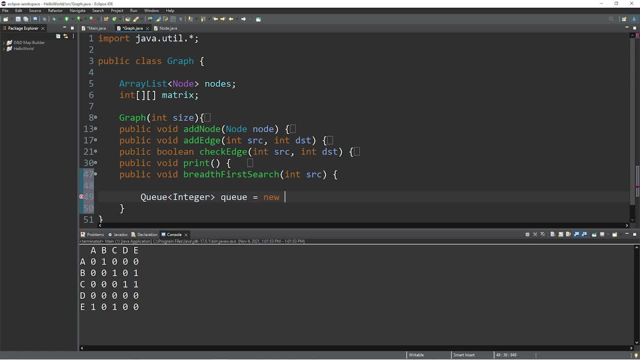 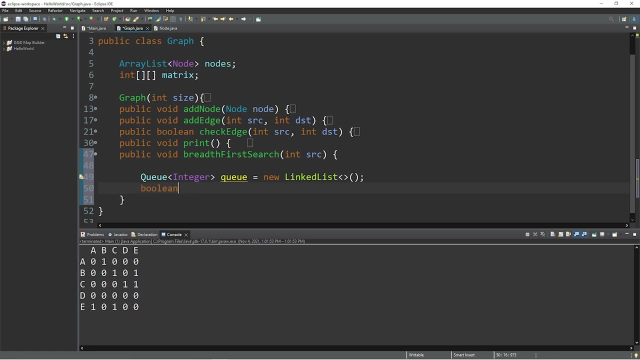 we need to use a data structure that utilizes the queue interface, one of which is a linked list. Okay, so we have our queue and we're going to create an array of booleans to mark if a node has been visited or not. So let's create a boolean array named visited equals new boolean. 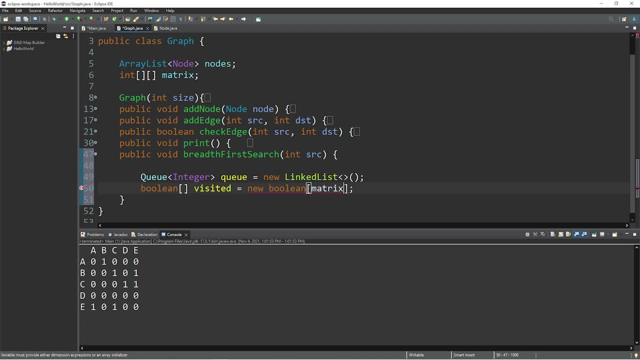 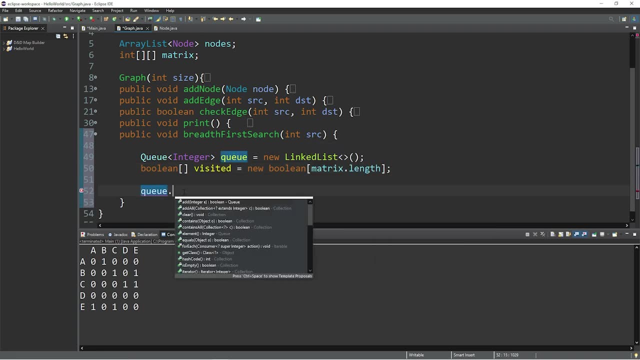 and the size will be matrix dot length With the node that we'll begin at. let's add that to the queue. Queue dot. you can use add or offer And then pass in the index of the starting node, Then within the boolean array of visited. 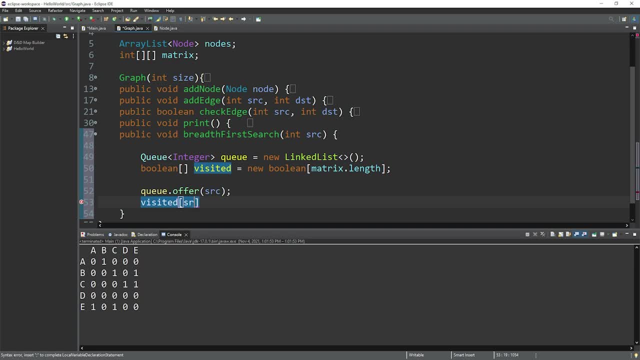 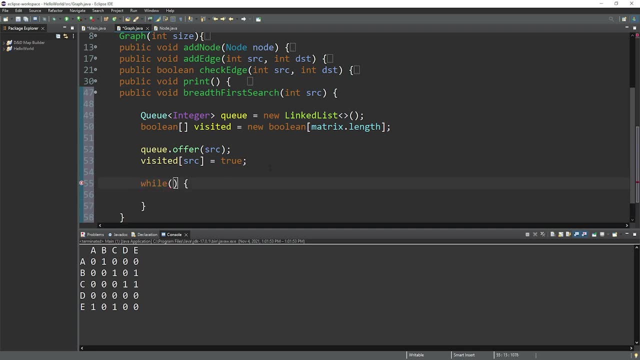 we will mark this as true At. index of source equals true, And now we'll need a while loop. Our condition is that we'll continue this while loop while the queue's size method does not equal zero. We'll assign our source equal to whatever is at the front of the queue. 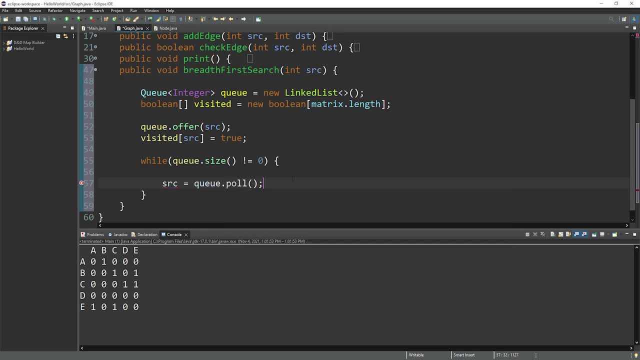 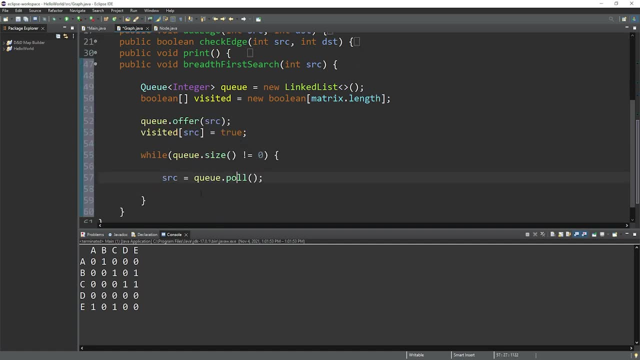 Okay, so now that we have the index of source equal to zero, we'll assign our source equal to the queue Queue dot. pull to remove an element. With this code that I've written, I've already went ahead and created an array list of the nodes to access the data Whenever we pull a node. 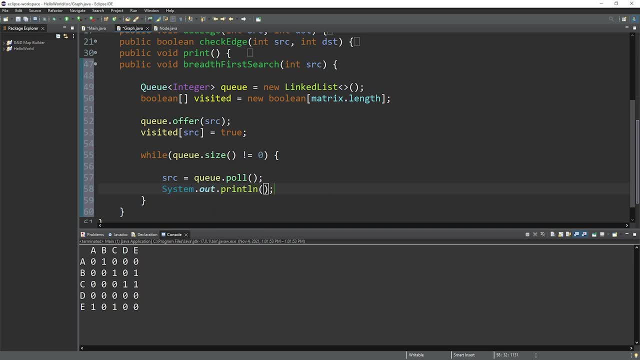 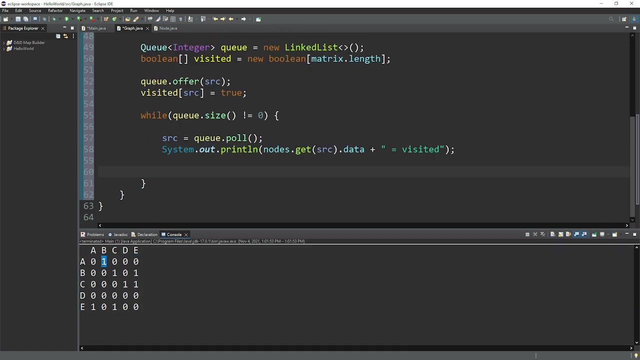 I'm going to display the data, So this part technically isn't necessary. Nodes dot get source dot data plus equals visited. Let's say that we're at node A. We're going to iterate over this row and look for any adjacent neighbors, So let's use 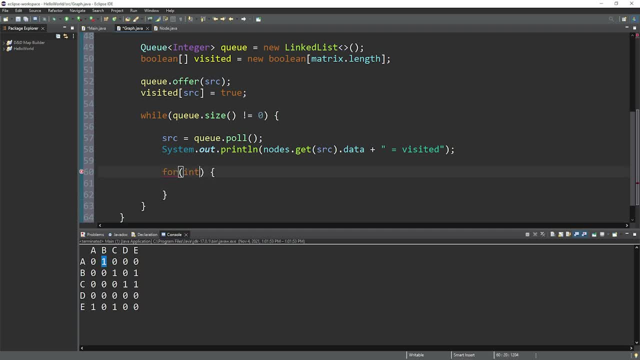 a for loop for that, For int i equals zero. We will continue this as long as i is less than our matrix at index of source dot length. This means the length of the row. Then i plus, plus. During each iteration let's check to see if this value is one and the node that we're trying to. 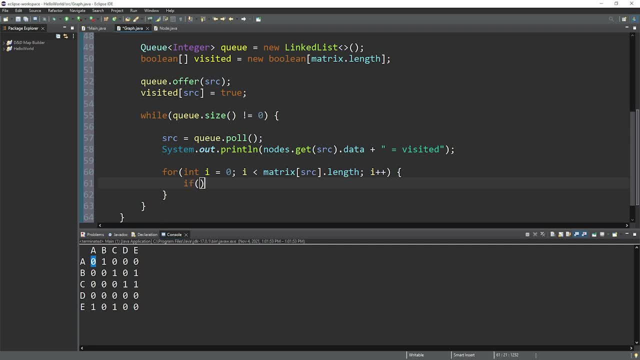 visit has not already been visited. If that's the case, then matrix at indices of source and i is equal to one, And visited at index of i is not true. So we can use the not logical operator If we have an adjacent neighbor. 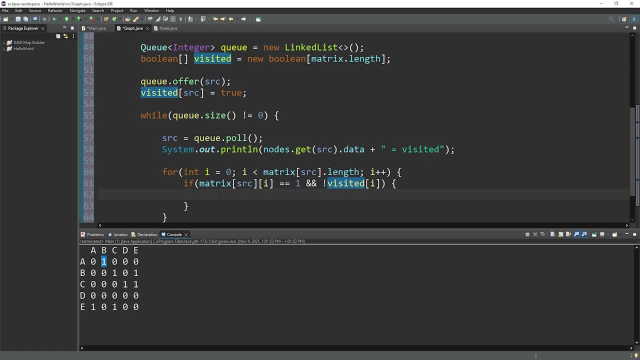 that's not been visited, then we will add the index to the queue And that node is going to wait in line. Queue dot offer. i And i is an adjacent neighbor, So we're going to add the index to the queue And that node is going to wait in line. Queue dot offer. i And i is an.